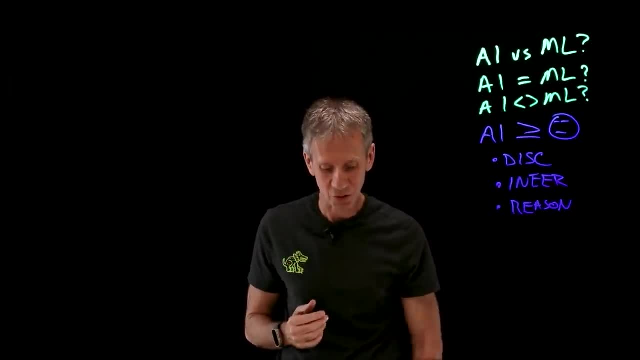 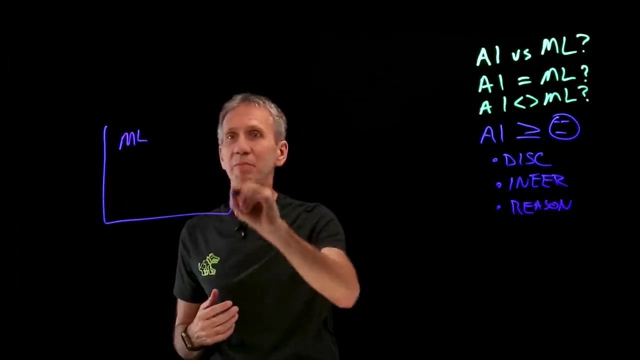 So I'm going to suggest to you: this is what AI is And that's the definition we'll use for this discussion. Now, what kinds of things then would be involved if we were talking about doing machine learning? Well, machine learning- I'm going to put that over here- is basically a capability. 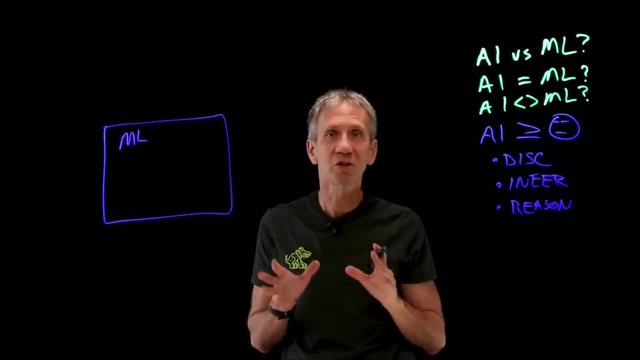 We'll start with a Venn diagram. Machine learning involves predictions or decisions based on data. Think about this as a very sophisticated form of statistical analysis. It's looking for predictions based upon information that we have. So the more we feed into the system, the more it's. 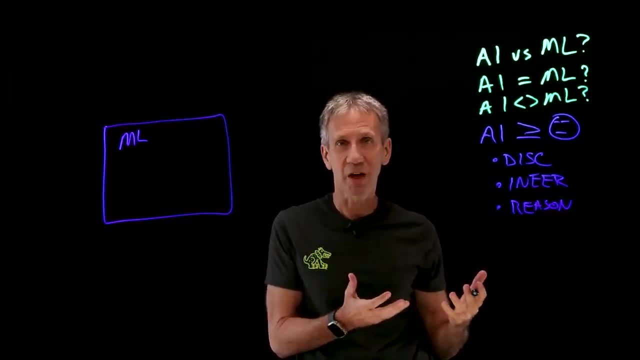 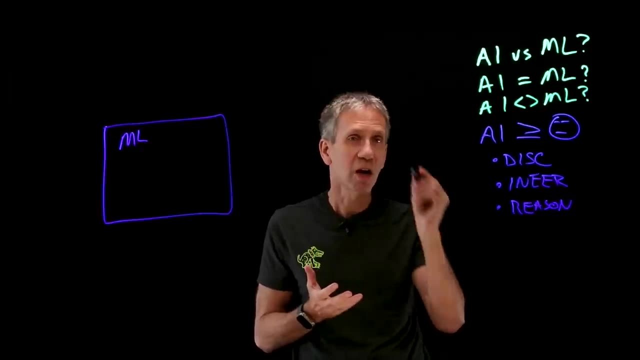 able to give us accurate predictions and decisions based upon that data, Then we have something that learns- that's the L part- rather than having to be programmed. When we program a system, I have to come up with all the code, And if I wanted to do something, 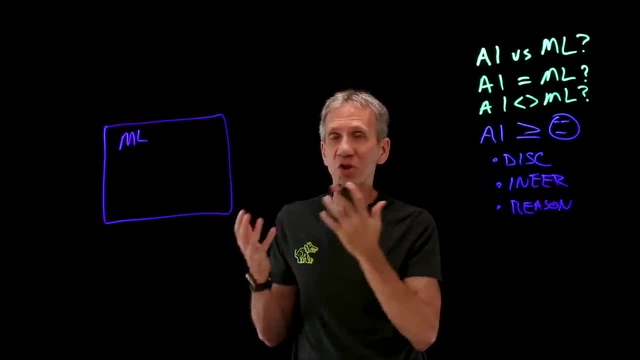 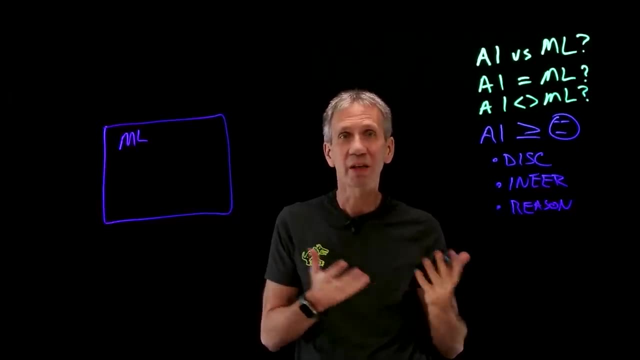 different. I have to go change the code and then get a different outcome. In the machine learning situation, what I'm doing could be adjusting some models, but it's different than programming And mostly it's learning the more data that I give to it, So it's based on large amounts of. 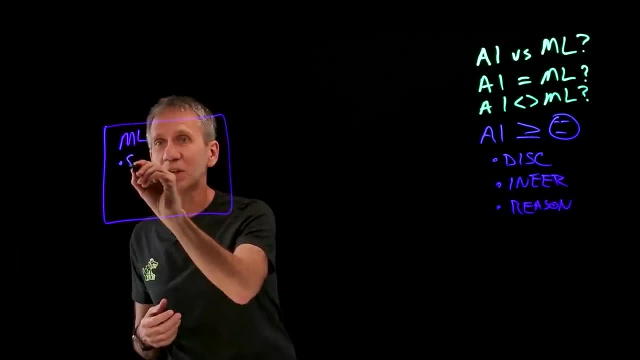 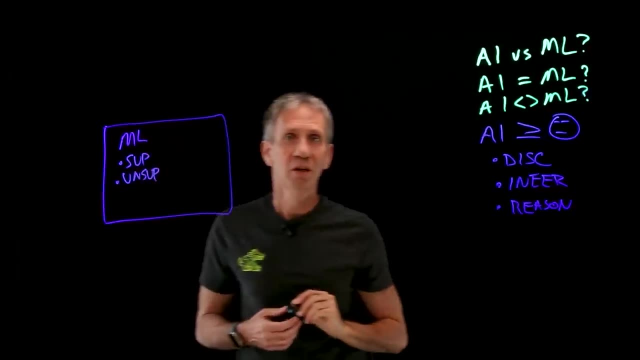 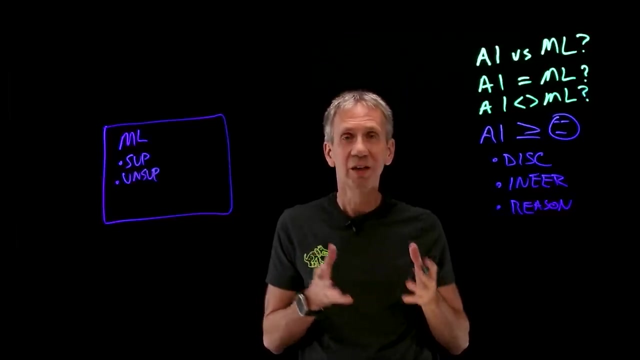 information And there's a couple of different fields within couple of different types. There is supervised machine learning And, as you might guess, there's an unsupervised machine learning, And the main difference, as the name implies, is one has more human oversight looking at the training of the data using labels. 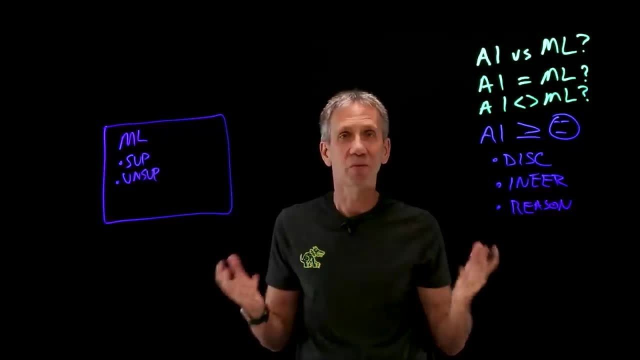 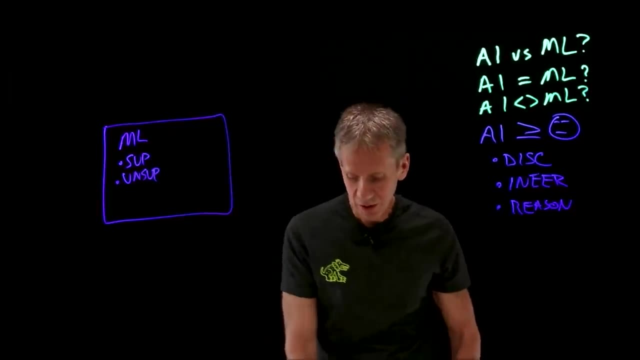 that are superimposed on the data Unsupervised, is kind of able to run more and find things that were not explicitly stated. OK, so that's machine learning. It turns out that there is a subfield of machine learning that we call deep learning. 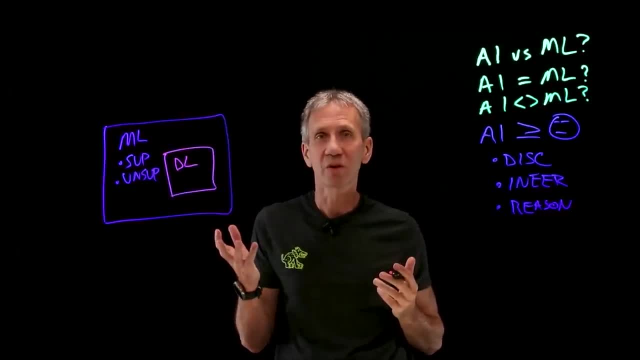 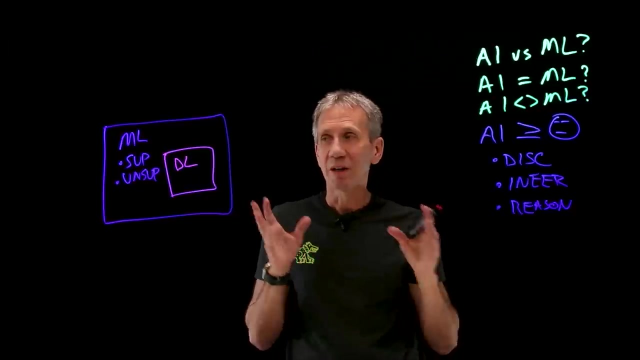 And what is deep learning? Well, this involves things like neural networks. Neural networks involve nodes and statistical relationships between those nodes to model the way that our minds work, And it's called deep because we're doing multiple layers of those neural networks. Now, the interesting thing about 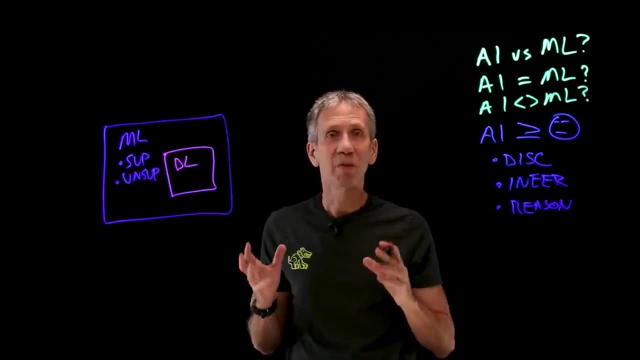 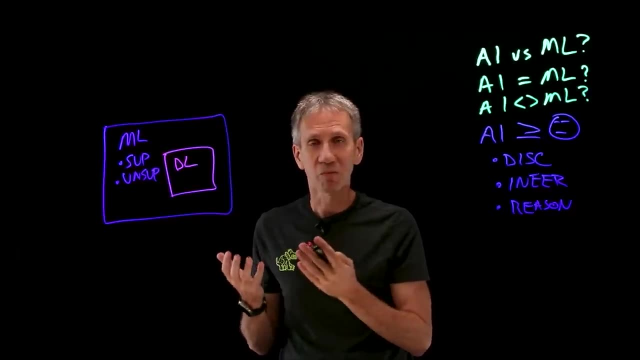 deep learning is. we can end up with some very interesting insights, but we might not always be able to tell how the system came up with that. It doesn't always show its work fully, So we can end up with some really interesting information. There's everything we know about the introspective network and the never changing 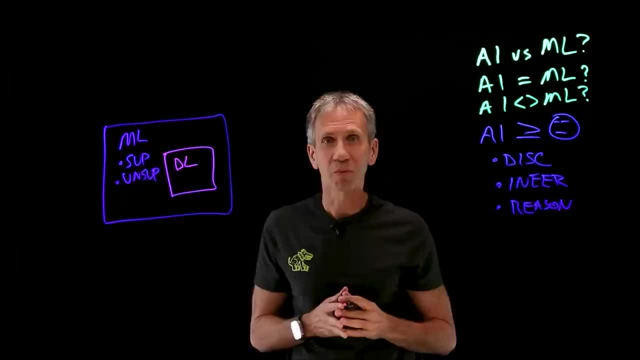 lya language. anything that's going out of the knowledge that we were all assigned to games and machine learning a time, how it works. So why does deep learning differ from science or science and what does deep learning differ? And yeah, I think that's one important place to look at deep learning. 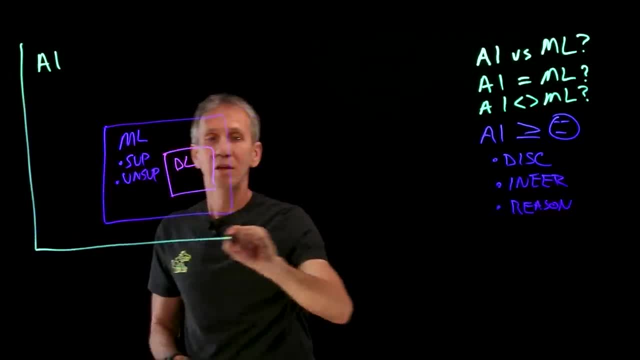 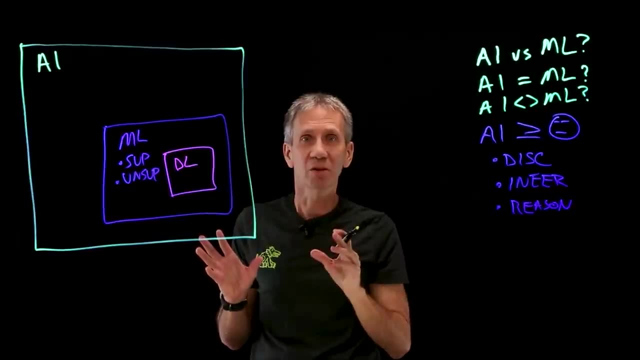 And then there are other things that challenge deep learning and again use data skills to did not even have to be challenged so strong. So let's try to keep moving with ourNovo organization. OK, Thanks a lot. Thanks again. Thanks, Thanks very much. 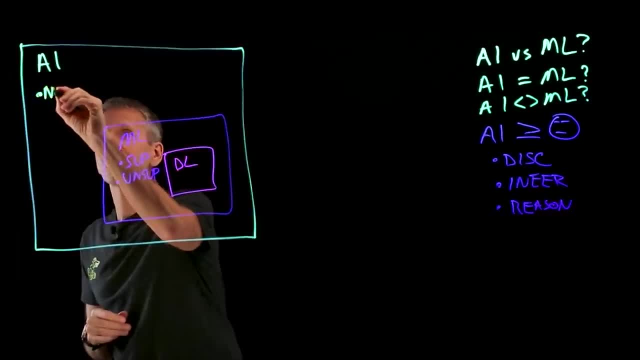 Thanks again. You should definitely stick a link, a link to the non-وف-the-talkcom bit of later video: click習op 구 mom�- other things be Well. we can involve things like natural language processing. It could be vision. 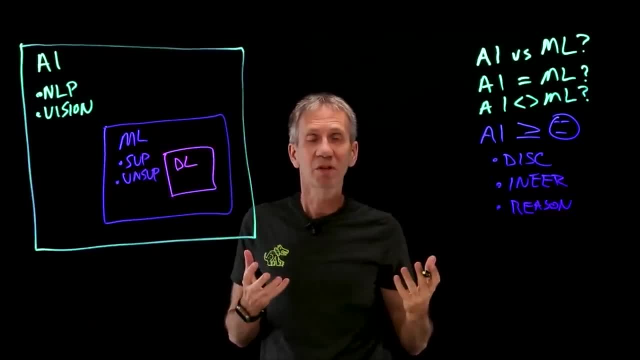 So we want a system that's able to see. We might even want a system that's able to hear and be able to distinguish what it's hearing and what it's seeing, because, after all, humans are able to do that, And that's part of what our brains do, is distinguish. 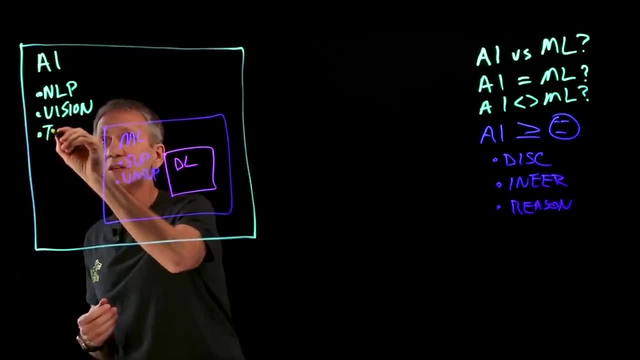 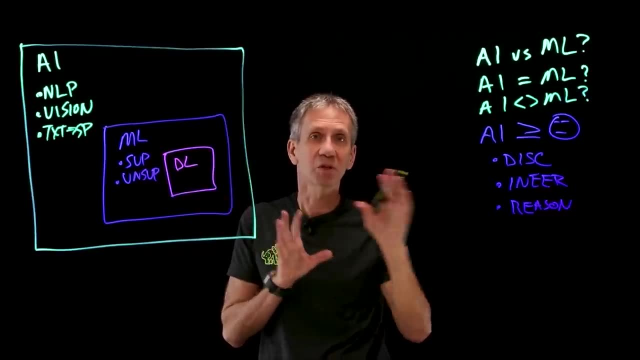 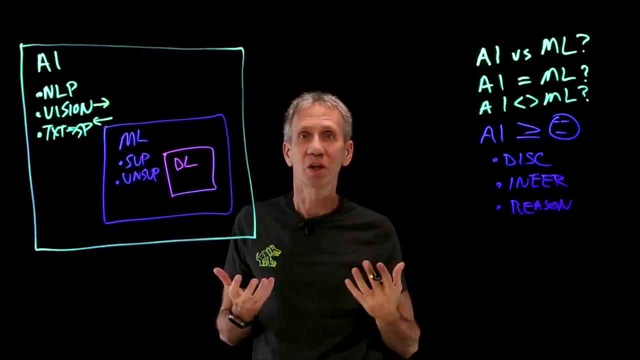 those kinds of things. It can involve other things like the ability to do text to speech. So if we take written words, concepts and be able to speak those out, So this first one involved being able to see things. This is now being able to speak those things as well. 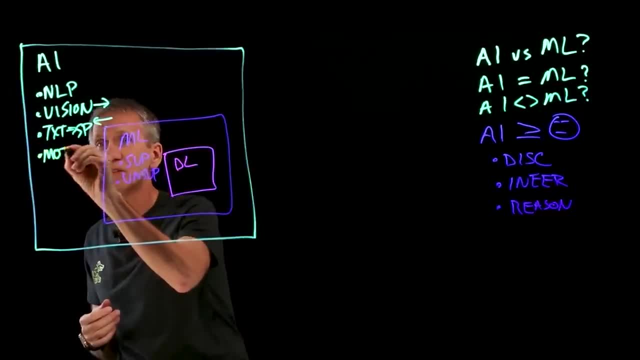 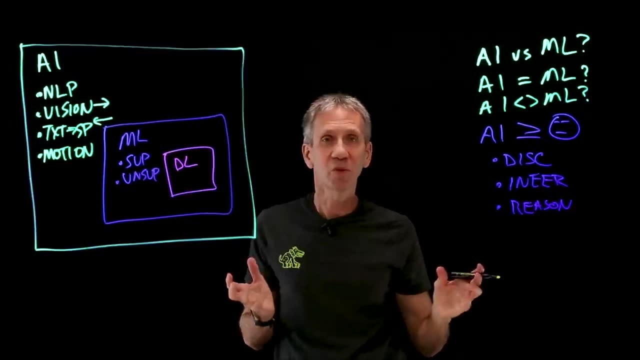 And then other things that humans are able to do. naturally, that we often take for granted is motion. This is the field of robotics, which is a subset of AI: The ability to just do simple things like tie our shoes open and close the door, lift something, walk somewhere, That's all. 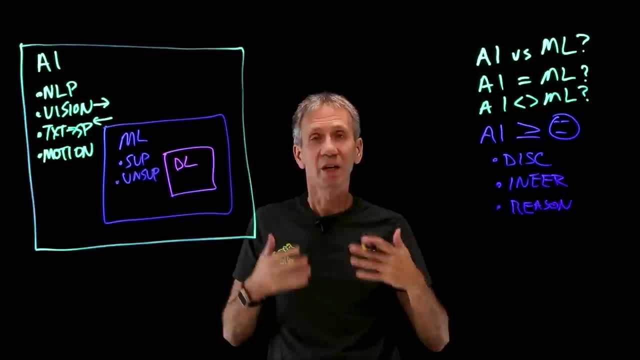 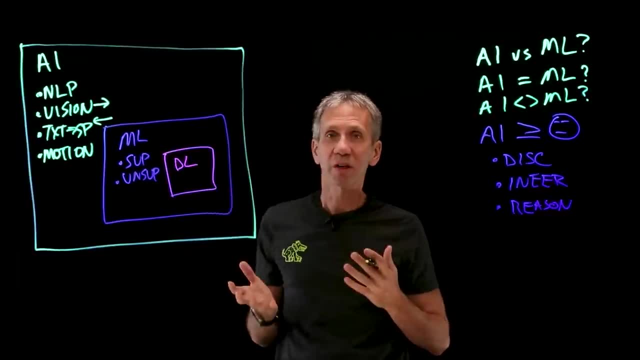 simple, Something that would be part of human capabilities and involves certain sorts of perceptions, calculations that we do in our brains that we don't even think about. So here's what it comes down to. It's a Venn diagram, and we've got machine learning, we've got deep learning. 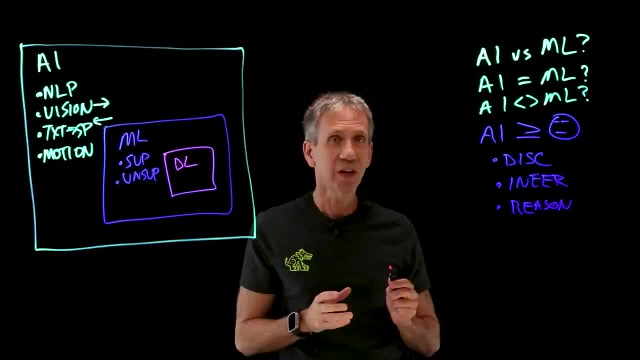 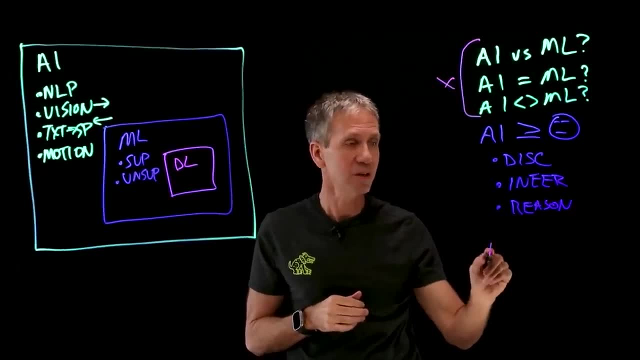 and we've got AI. So I'm going to suggest to you: the right way to think about this is not these equations. Those are not the way to look at it, In fact, what we should think about this as machine learning is a subset. 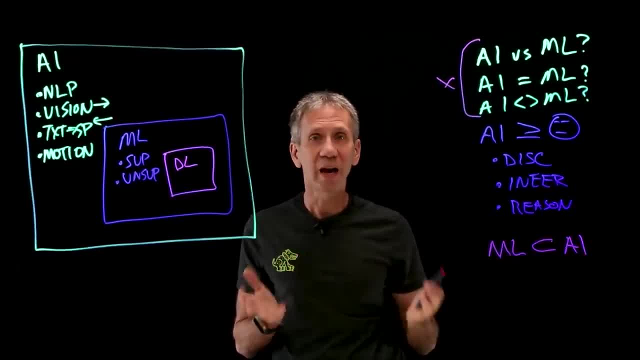 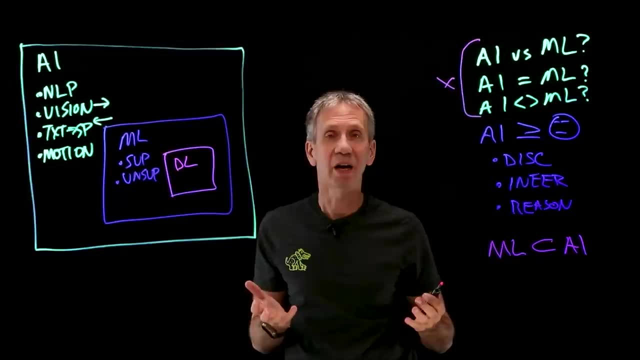 A subset of AI, And that's how we need to think about this. When I'm doing machine learning, in fact I am doing AI. When I'm doing these other things, I'm doing AI, But none of them are all of AI, but they're a very important part.